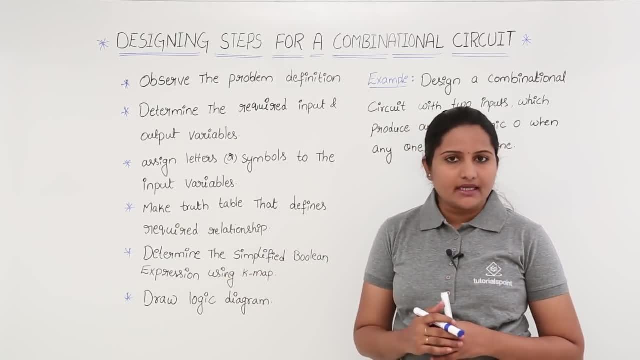 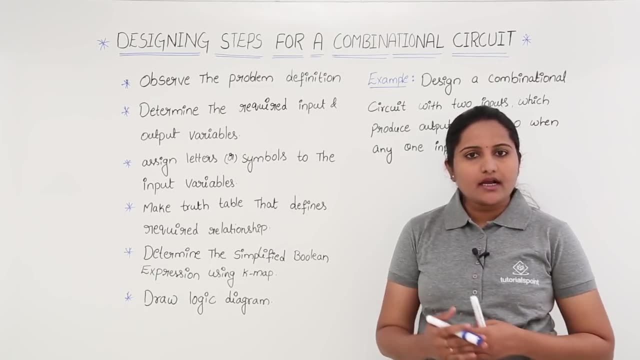 So next, determine the simplified Boolean expression using K-MAP. So you know that, for example, if you are having a truth table. So you know that, for example, if you are having a truth table for a functionality, you can draw K-MAP for that. In K-MAP's concept we discussed that how to. 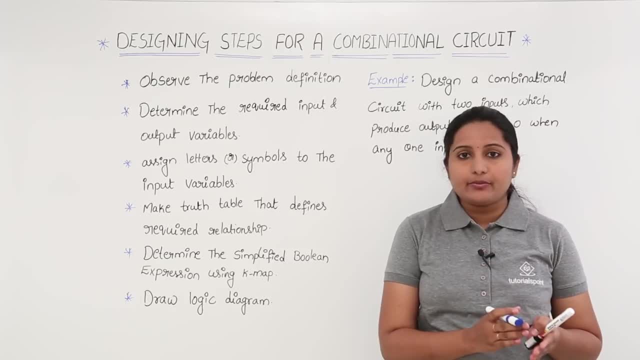 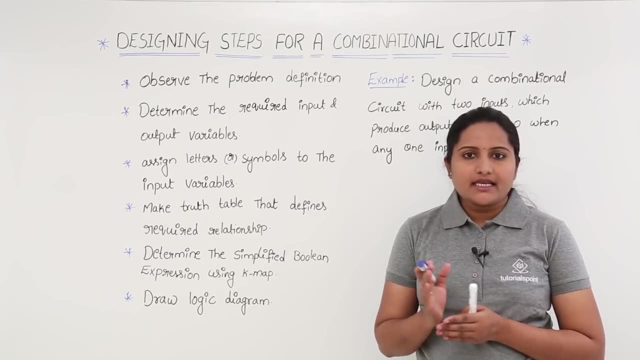 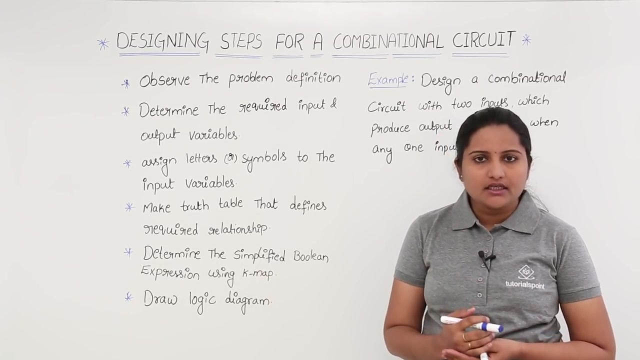 draw a K-MAP from truth table. In so many example problems also we draw like that from truth table to K-MAP. From K-MAP we are obtaining the expression related to the functionality. So by using this K-MAP from truth table we are getting the required relation equivalent Boolean algebraic expression. 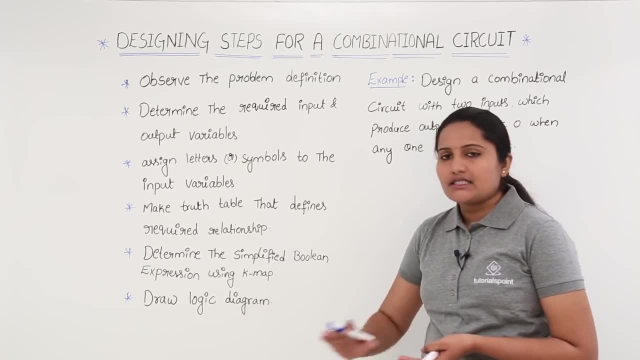 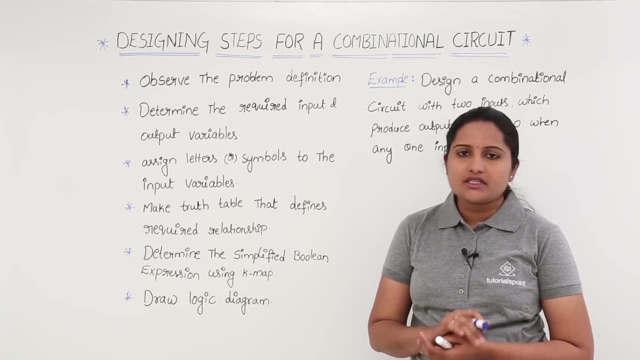 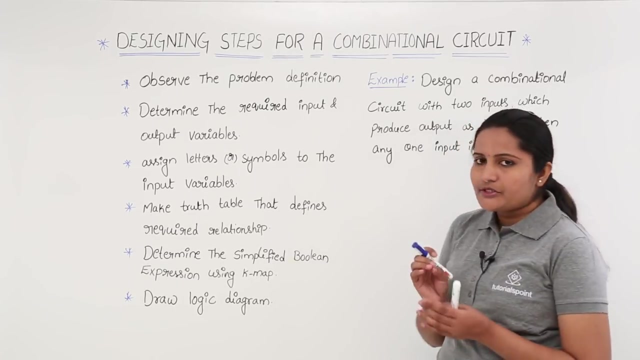 By using that Boolean expression you are going to draw the logic diagram using logic gates. So these are the main steps included in designing a combinational circuit. This is very, very important throughout the combinational circuit designing concept. So here observe the problem definition. 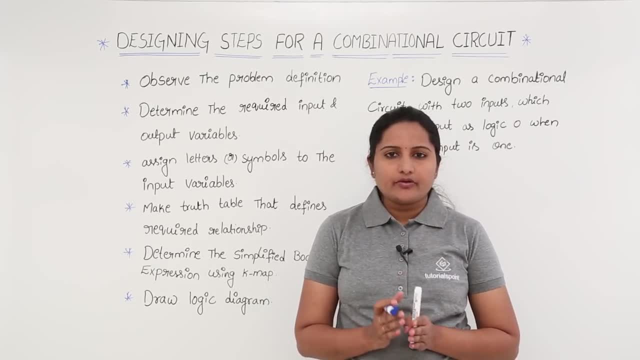 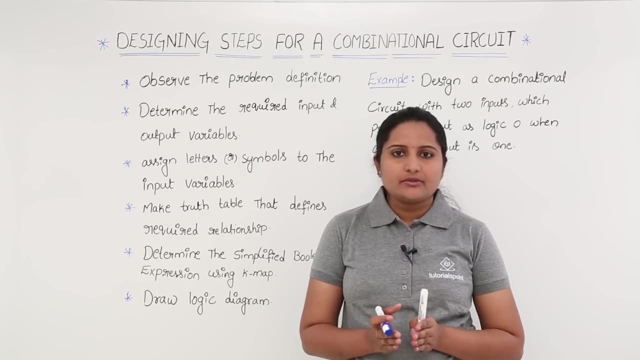 and then determining how many input and output variables are required and naming that input output variables and after that considering the truth table for required relationship, after that K-MAP for the truth table for getting Boolean expression. finally, logic diagram. these are the steps. Now, for example, I am considering a small 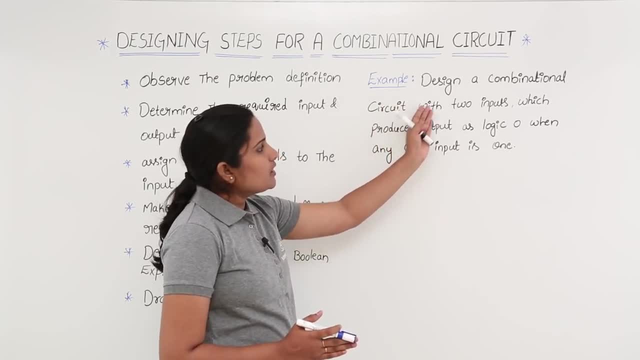 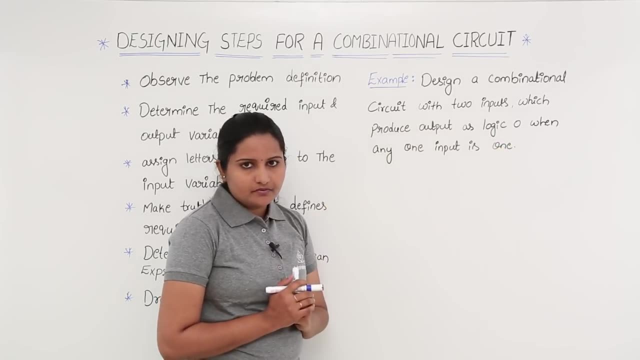 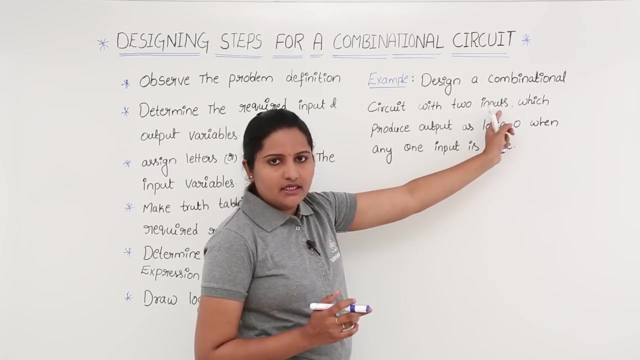 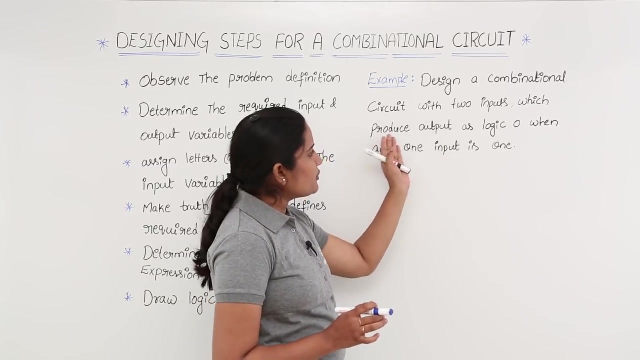 problem. So design a combinational circuit with two inputs which produce output as logic 0 when any one input is 1.. This is my problem statement Here. they given design a combinational circuit with two inputs Initially. your problem is stating: you are having two inputs, So definitely, which produces? 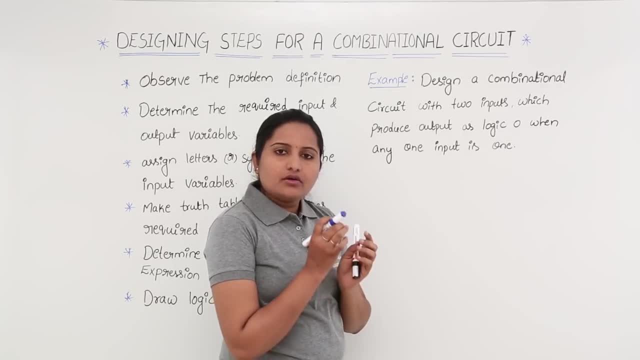 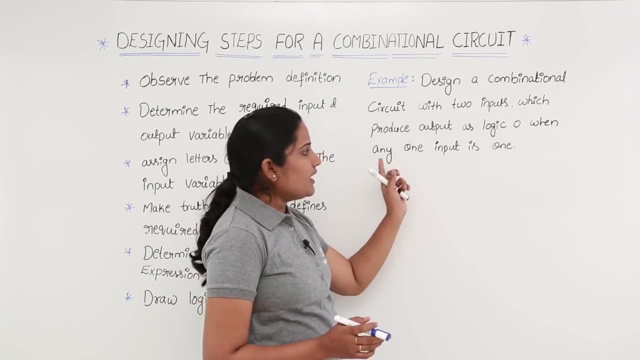 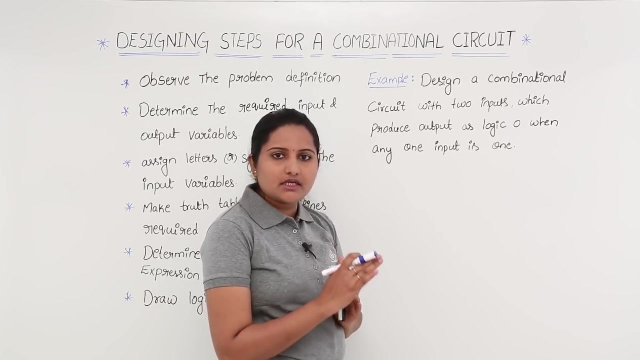 output as logic 0. so that means so whenever you are having two inputs, your output is producing logic 0, when any one input is 1.. In that two input combination, if any one input is 1, you are circuit must produce so logic 0. So that means the output is producing logic. 0.. So if two inputs are present, there is a natural output when the second circuit is producing logic 0.. This function is nepal 4000, Innovative combinational circuit. ok, in short, that means all the inputs are mystical, It is all logical. Well, so let me paste with this solutionCheck. 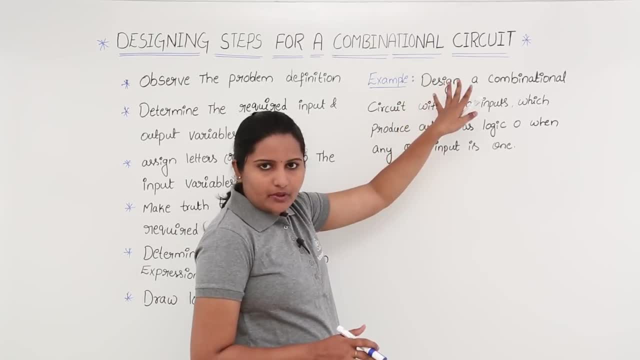 Put these two��啊and Galaxy out, we will get the rhyme and then the other solution. So let me use shape output, which is simple. So that means the output. the Hmše yang yani is 1 here. So after observing this problem, you understood the. so here you are having 2 inputs. 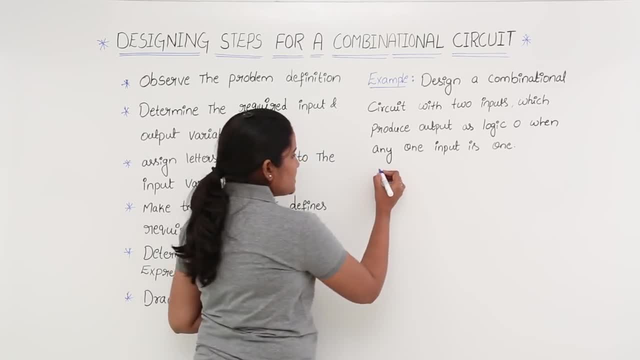 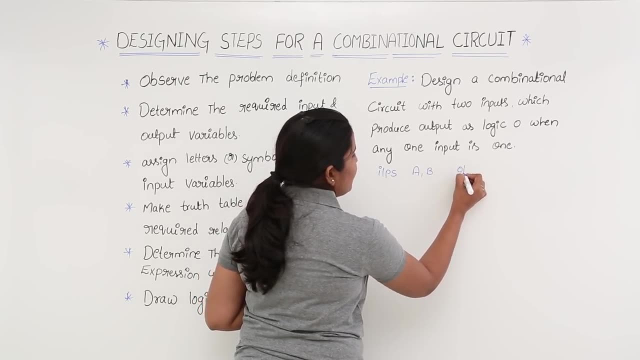 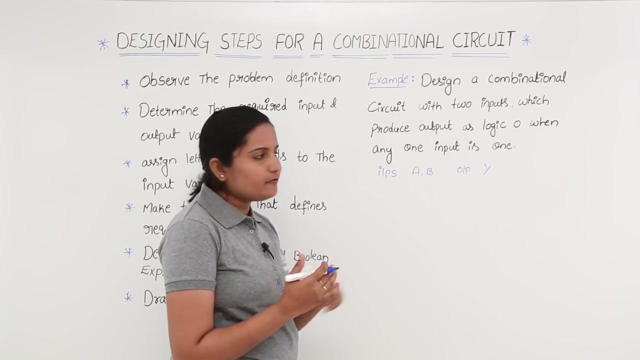 and 1 output. I am naming the 2 inputs as so. here the 2 inputs I am taking as a, comma b, and output I am naming as y. After naming this input and output variables, our aim is to draw the truth table for this relation, to satisfy this relation. Now I am considering truth table. 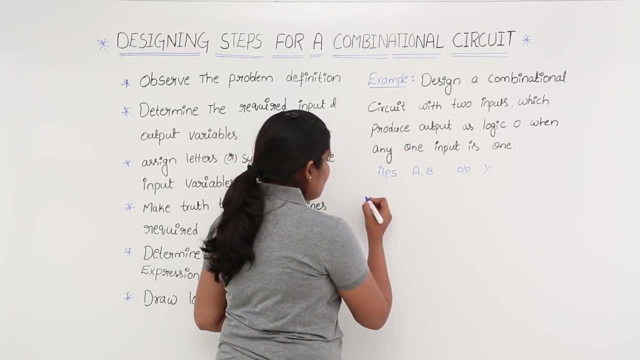 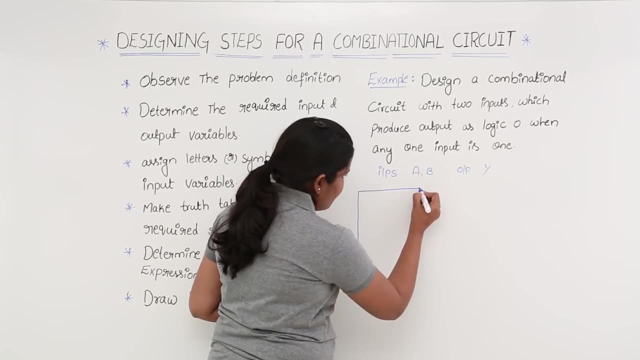 for this problem statement. So the truth table always contains input and output variable. as I already told you, when we are discussing truth table concept, First of all we need to consider input variables and after that output variables. in a truth table, Here you are having 2 inputs. 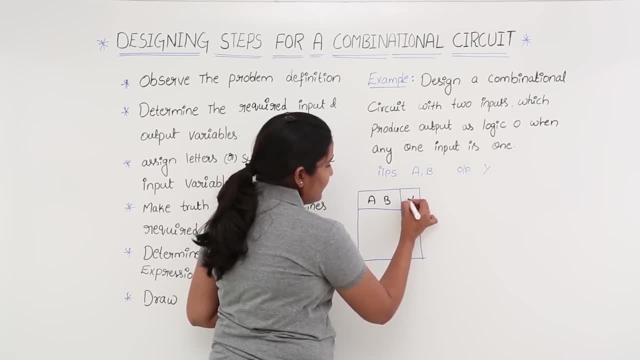 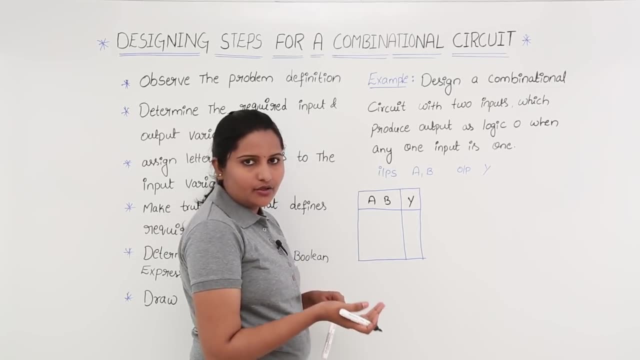 a and b and 1 output. you taken like y here. So now with 2 inputs, how many input combinations may be there? You know that 2 square combinations may be there. For example, if you are having 3 inputs, you may have 2 cube combinations Here for 2 inputs you may have 4 combinations that. 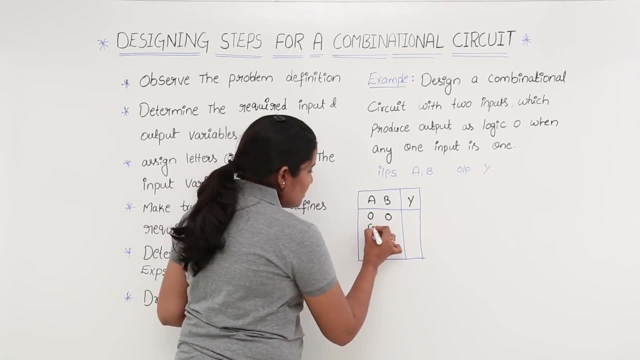 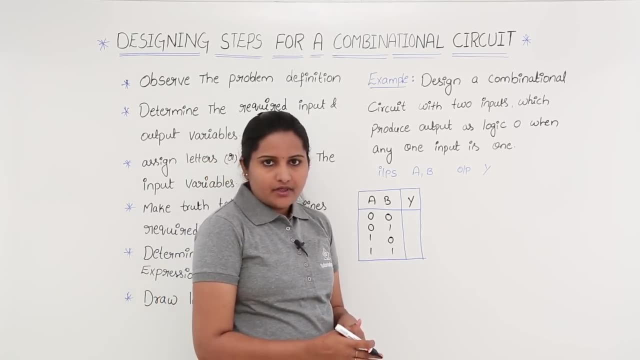 4 combinations I am considering like 0, 0, 0, 1, 1, 0 and 1, 1.. So, after considering the truth table, I am considering 2 inputs, a and b, and output. you considering input combinations. So why we are considering input combinations means when 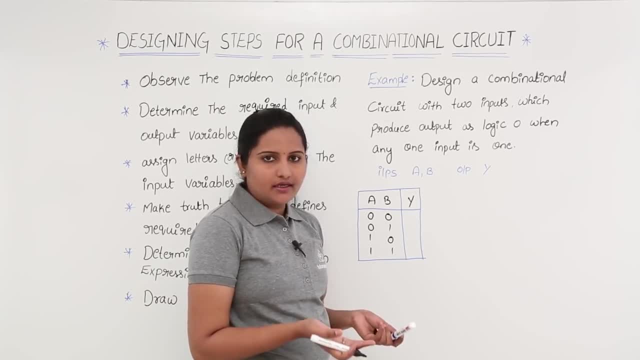 we are giving input to a circuit, we need to give in combination only. For example, A is sometimes 1, A is sometimes 0, B may be sometimes 0, B may be sometimes 1.. So we need to consider all combinations, all possible combinations for that circuit. So then only, for example: 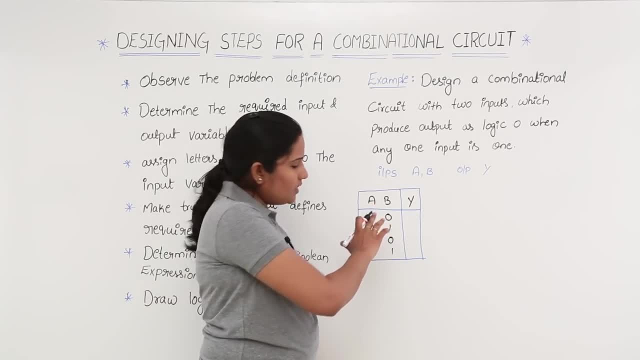 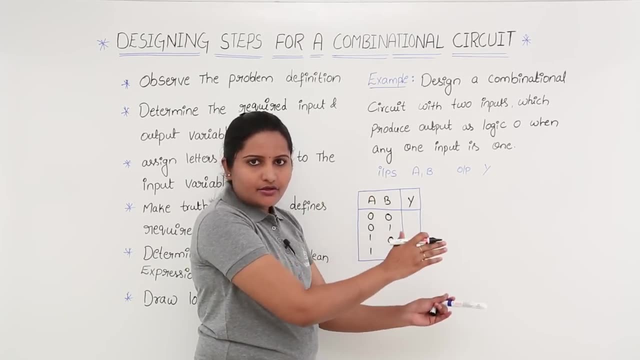 if you are not, if you are not taking all combinations in truth table, whatever circuit you are going to design, with any miss of combination, that is not going to provide for missed combination, that is not going to provide the output for missed combination. So this is only the problem. 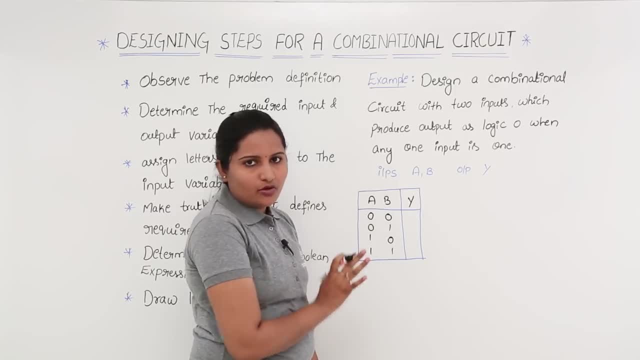 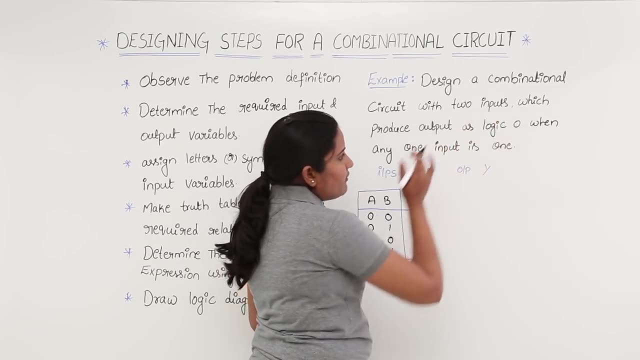 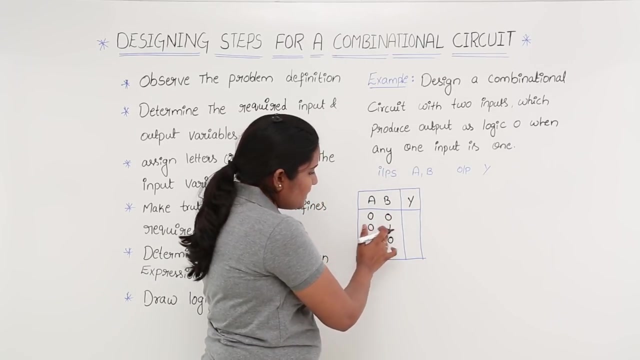 here. So now we considered all possible combinations here. So now what our problem stating is: it is going to provide logic 0 when any one input is 1.. So any one input is 1 means here is: any one input is 1, here also any one input is 1, and here also 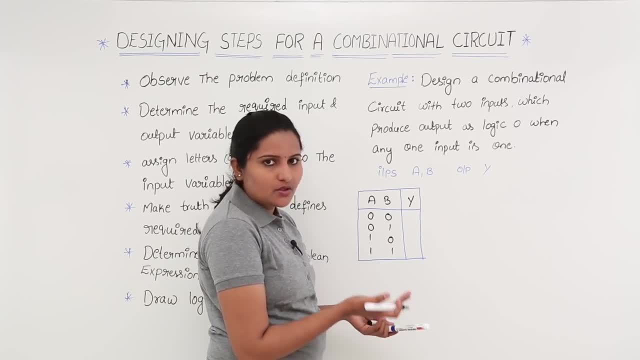 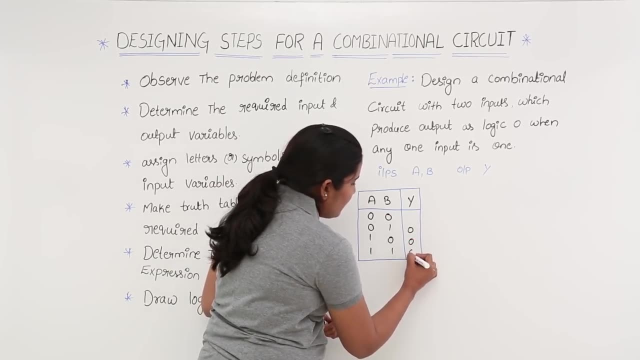 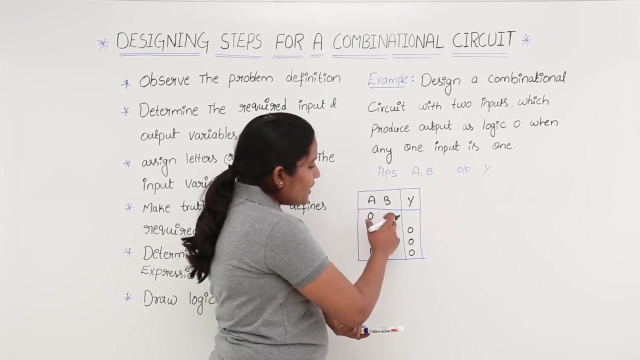 any one input is 1 means two input, two inputs also one will also come under same situation. So here our circuit need to provide 0 at out. So whenever at least one 1 is there in the input combination, So whenever you are not, 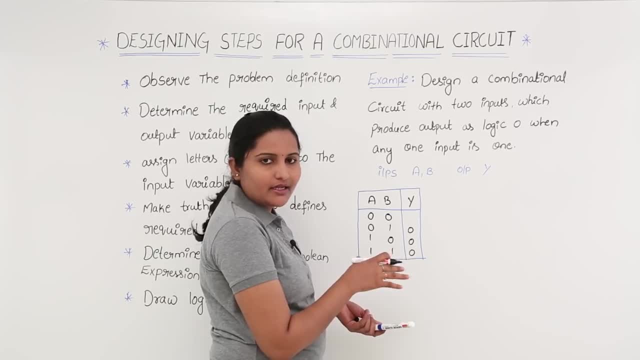 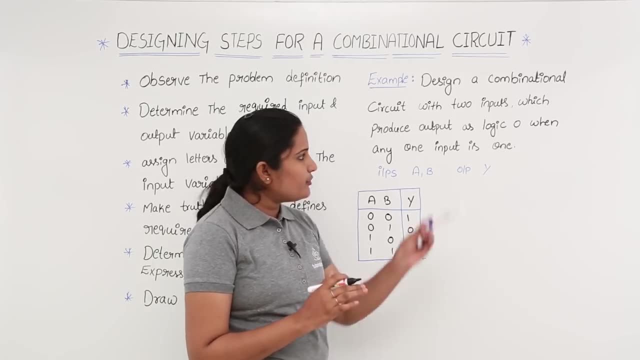 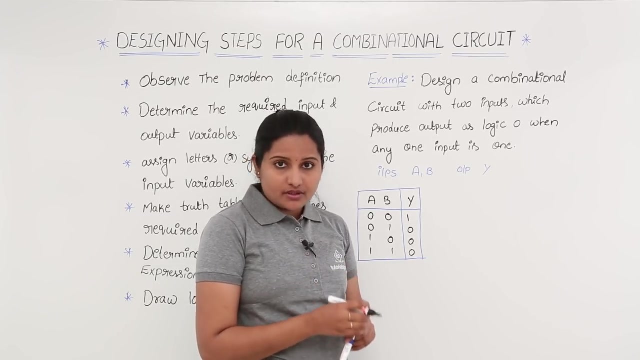 having at least one 1 in input combination. definitely your circuit is going to provide 1.. So you design the truth table for your required relationship. So after that, the next step is to design a K-MAP. Now you need to decide. you require the Boolean expression. 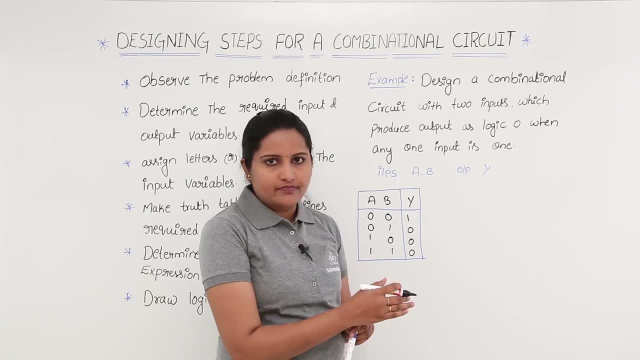 from K-MAP in product of sums or sum. So you need to decide the Boolean expression from K-MAP in product of sum of products. For example, if you want your Boolean expression from K-MAP as sum of products form- that means SOP form- you need to consider 1s in the functionality. 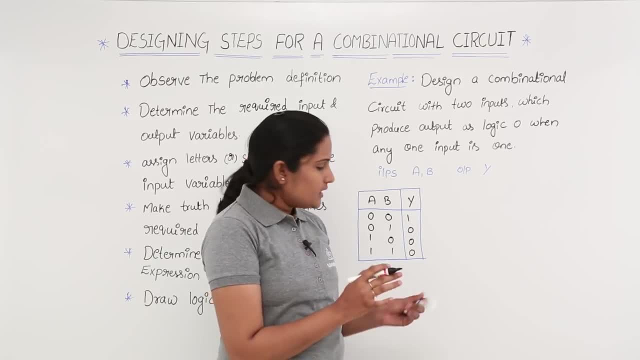 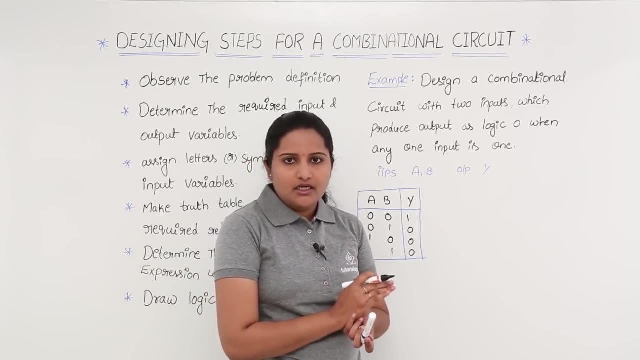 If you want in POS form. that means product of sums form. definitely you need to consider 0s in the truth table. So now, generally we will consider sum of products only. So I am going to consider sum of products. that means 1. I am going to consider for K-MAP. 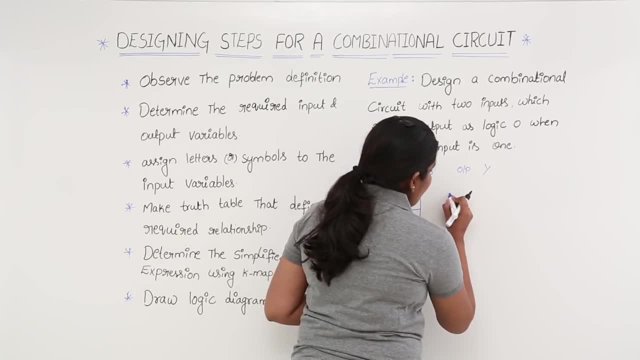 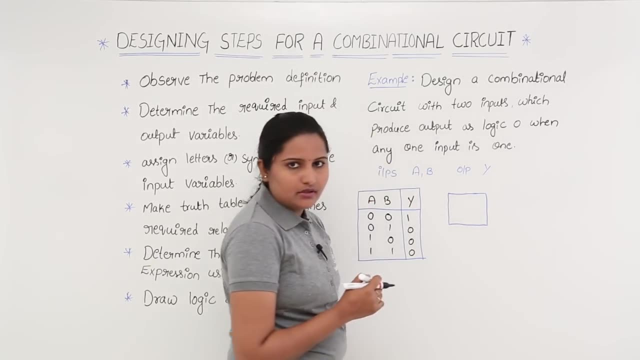 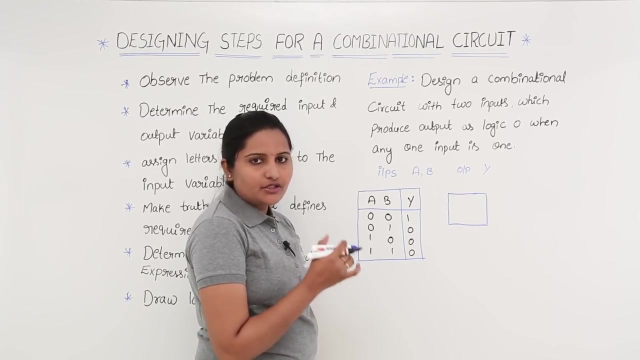 K map. So I am taking K map here. So how many variable K map we need to consider that can be designed by decided by the input variables. So how many input variables we are having here? 2 input variables we are having, So we are going to consider 2 input variable. 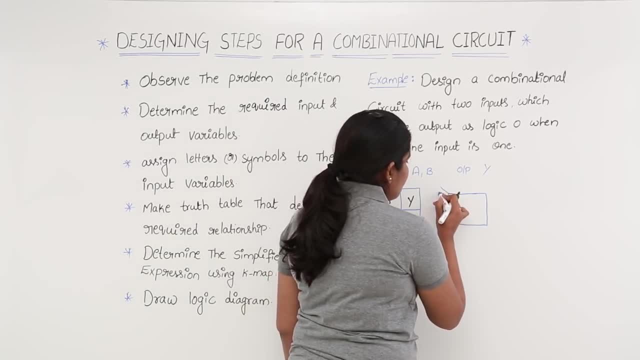 K map. So here 2 variable K map. I am considering: here I am having A and here I am having B. for this A, B. So the combinations are 0, 1 and 0, 1.. Now see here where you are having. 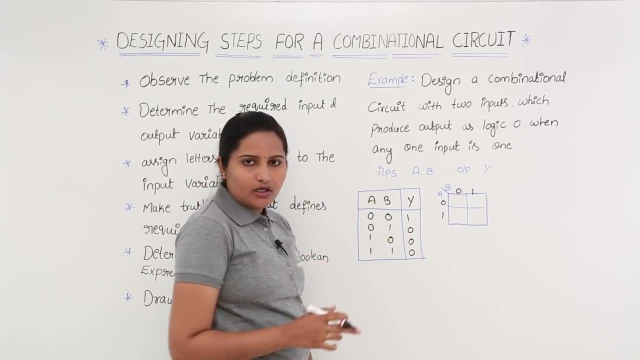 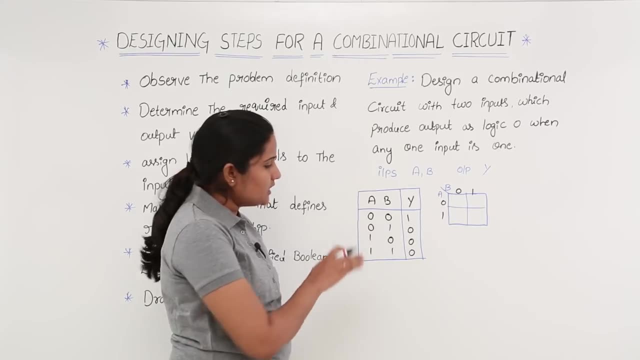 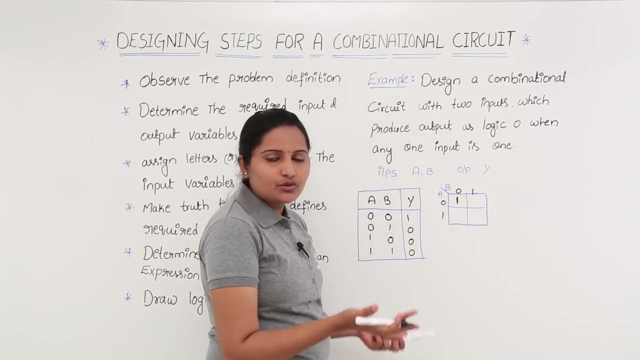 1. whenever A equal to 0, B equal to 0, then only your functionality is 1. in all the cases your circuit need to provide logic 0. So here you are placing 1.. Now there is no other ones to group as a double or quarter or octet. 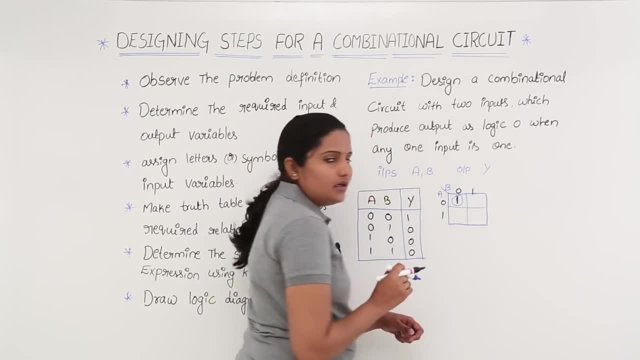 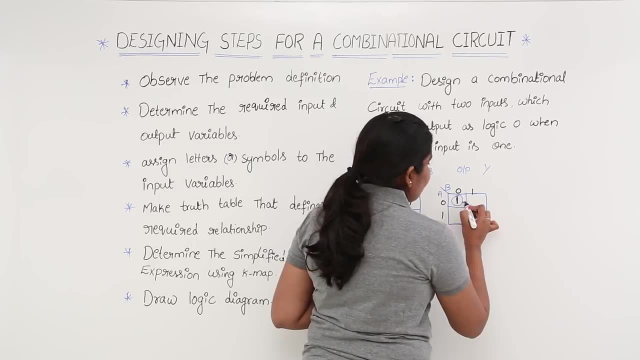 So you are placing 1.. Now there is no other ones to group as a double or quarter or octet, So you need to group this single one and this is a one and only prime implicant in that K map which produces the Boolean expression. Now you need to consider the value equal. 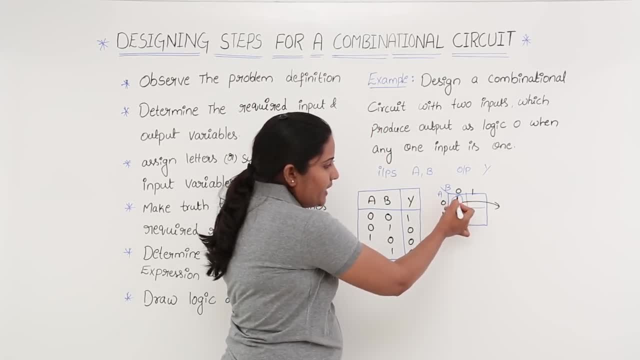 to that prime implicant. You just see, for this grouping, this is covering only single cell. So that is why, whatever value is there that you need to consider as it is, you can see top wise So that in top wise also, it is covering only single cell you can take. 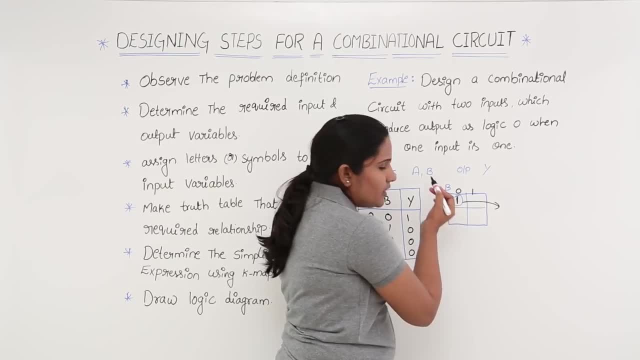 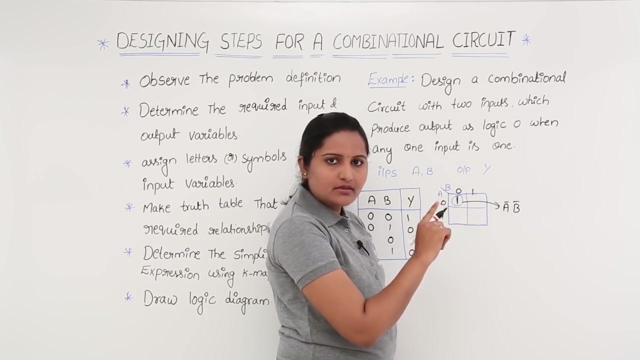 as it is. So here you can see that. you can see that here, side wise 0, this 0 represents A. whenever SOP form 0 represents A means you need to consider as A bar. So A bar, B bar. So top wise 0 representing B, So 0, B means B bar. 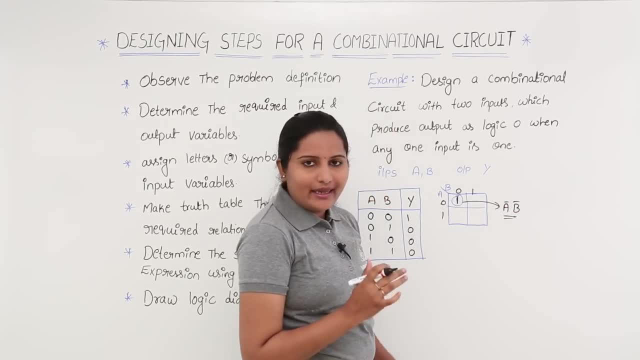 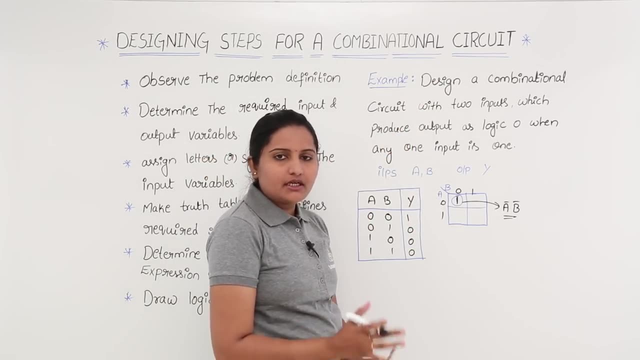 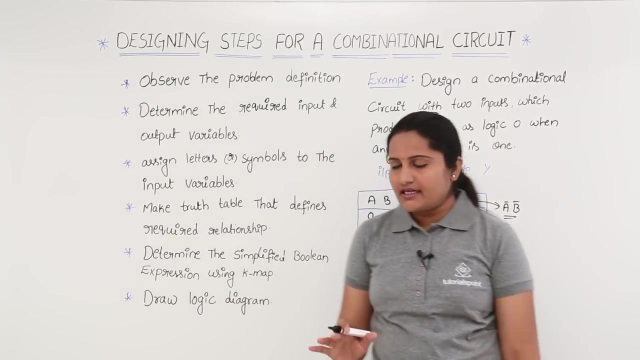 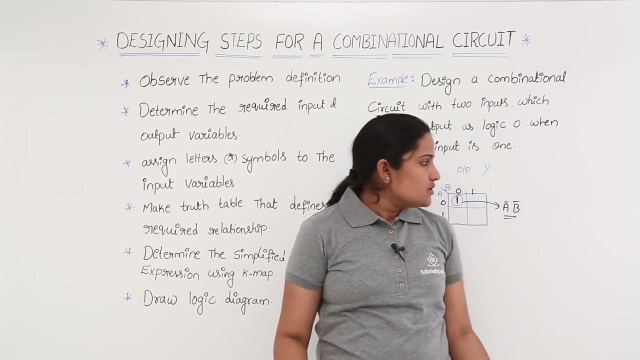 So A bar, B bar is the Boolean expression came from this K map. So, whatever your required functionality is there, the Boolean expression relating to your functionality, Your required functionality, is A bar B bar. and we are in now final step, that is, draw the logic diagram according to the this K map expression given. So here you have got. 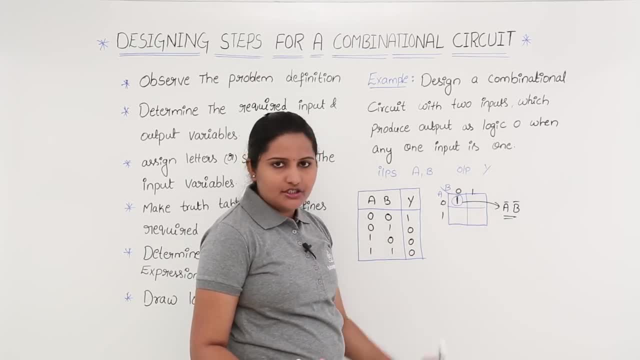 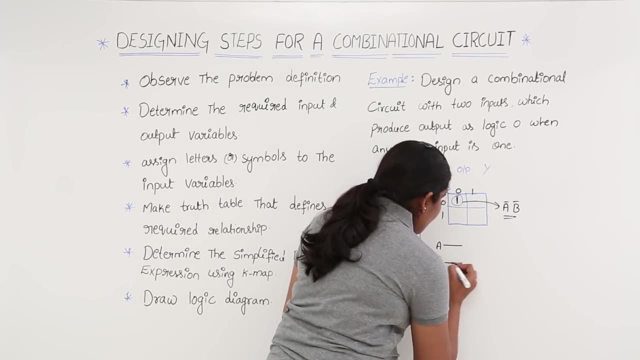 A bar, B bar as your resultant K map expression for this relation. Now I am drawing truth table. for example, if you are having A at input side and B at input side, Now for this A, I am taking a non-coherent half of the model. So for the non-coherent of the model, I am 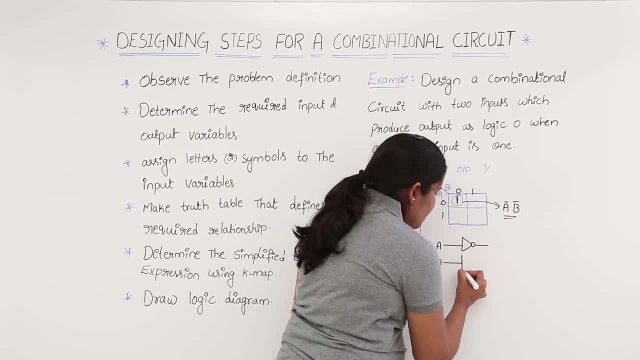 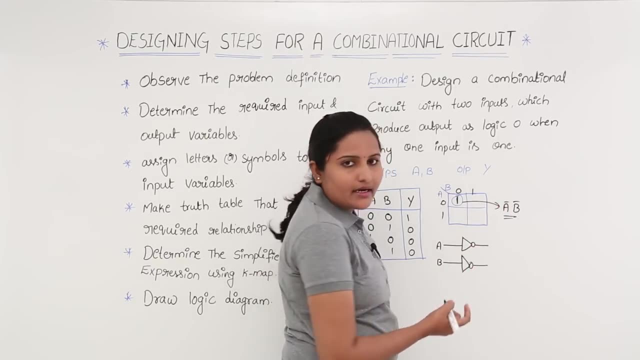 taking a non-coherent half of the model. So when you are taking either the two variables not gate, and for this b I am taking a not gate, another not gate here. why? because I require a bar and b bar. So to get a bar and b bar, I am taking two, not gates here, and then you need to.